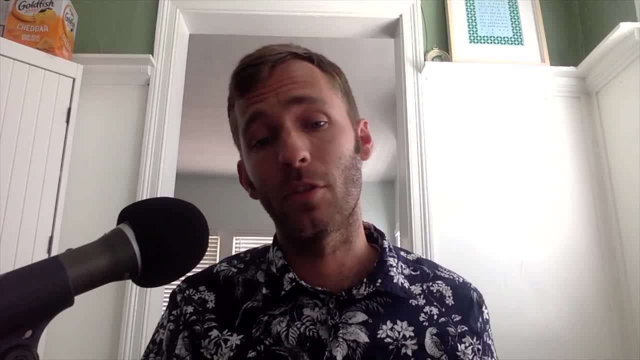 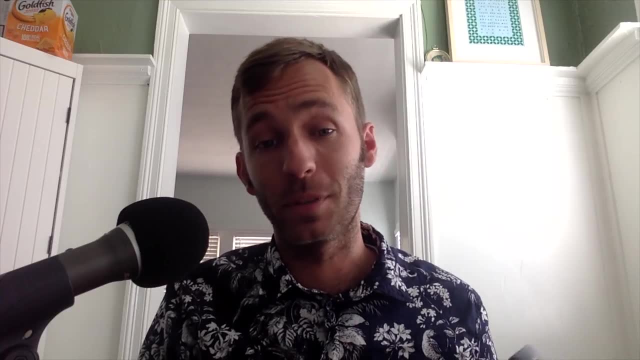 uploading a simple card game. There are so many other tutorials on the Game Crafter's website for different things, but I suggest that you actually just kind of walk through, browse their website to see all of the different sort of game elements that they have. You can. 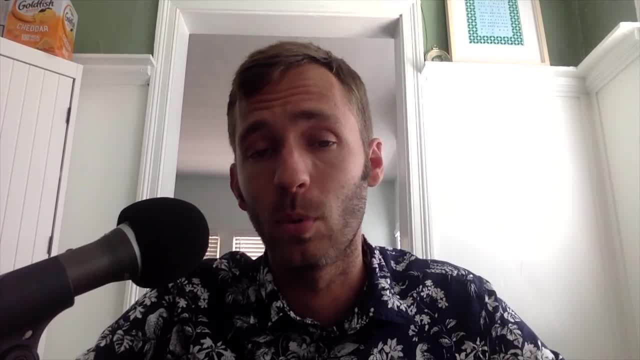 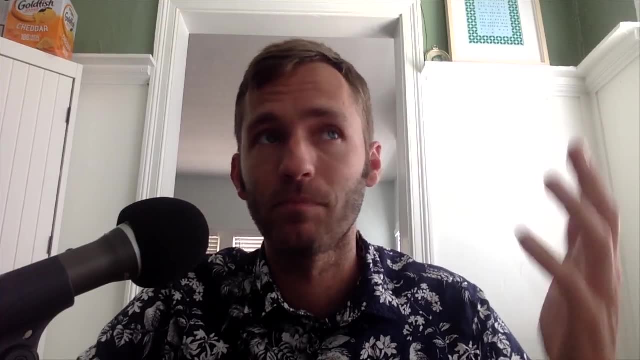 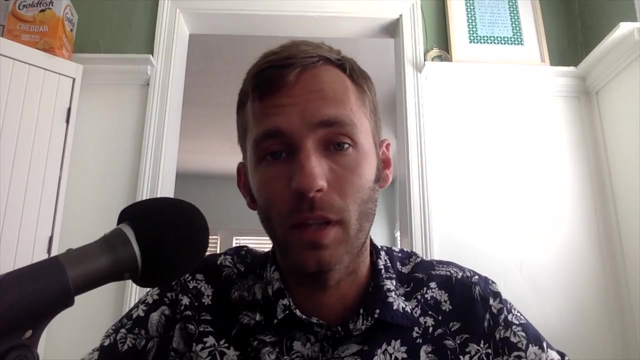 really build almost anything you want to do from card games, board games, games with dice and pieces and miniatures. There's so much I can't even wrap my mind around everything that's there so kind of. they have tons of great tools that help you calculate what the cost of it's going to. 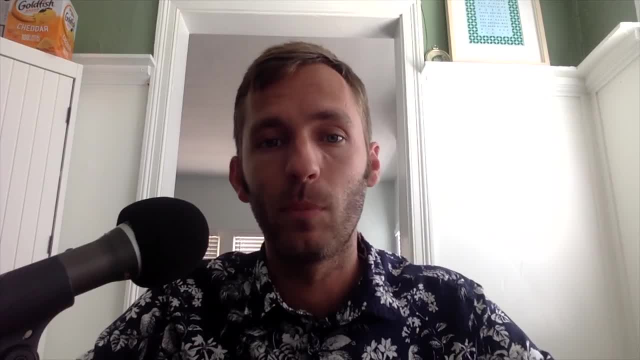 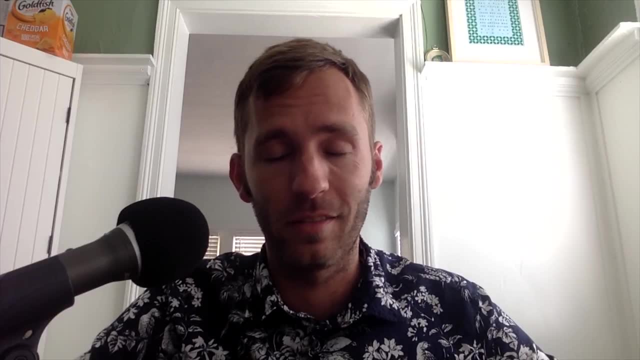 be and you kind of just build the game with these different pieces and upload all of your files there. It's really easy. They provide you all the specs and the sizes for those and, yeah, it's incredible. So Triumvirate is a card game. There's a 90 card deck here. This is called their. 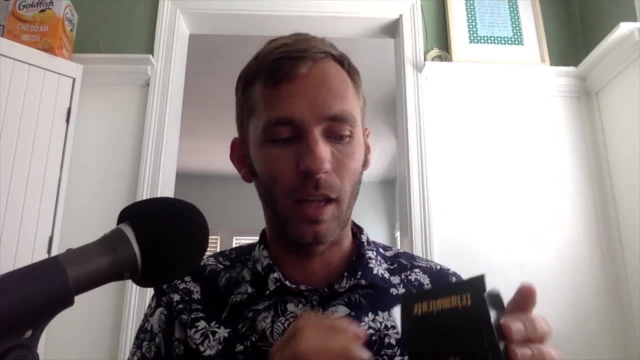 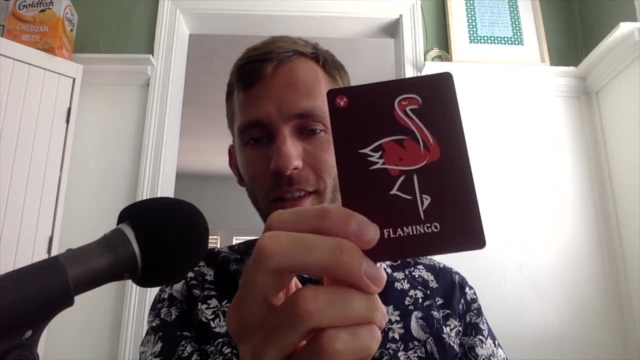 Tuck Box, which this is like something you would just find in a game store. so my cards are in. here They are- This is a fun one, You know, based on Kingdom of Florida, so there's some characters, animals, but these are like. 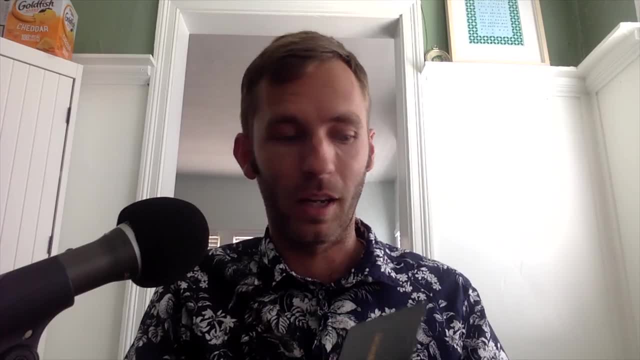 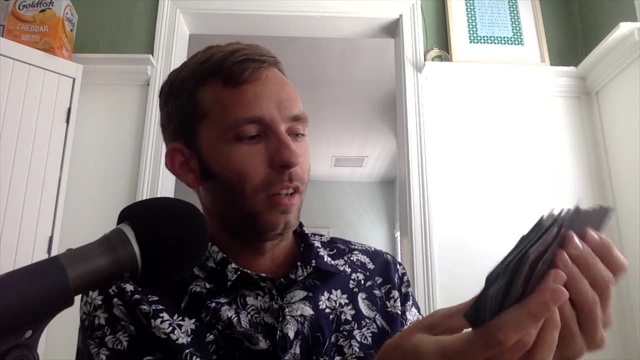 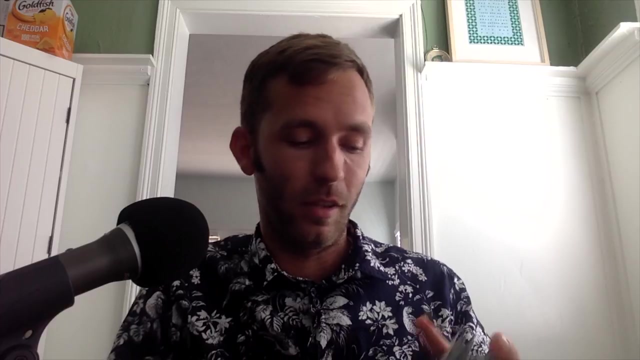 legit quality like a normal card deck that you would find in any other game. Just a quick sneak peek: There's a lot of fun like colorful things in here, and this is based on my book series, but you don't have to have read the series to play this game. 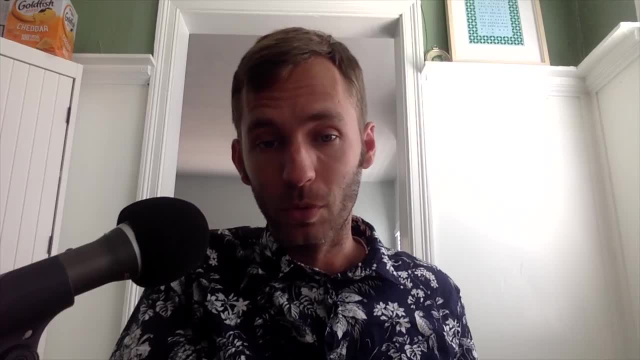 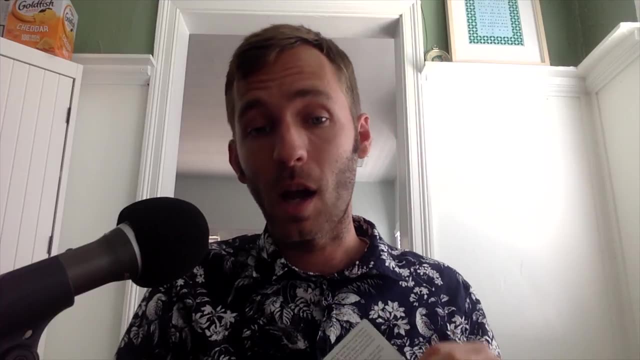 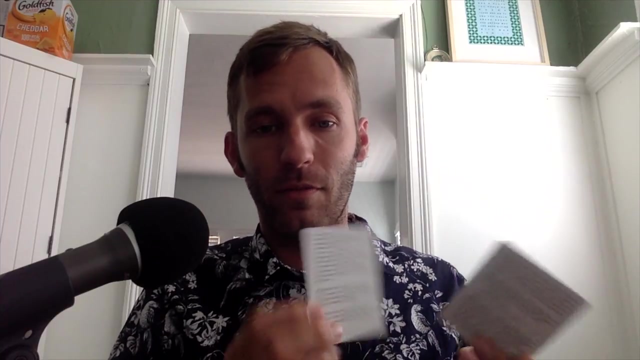 I also used two of the cards to print the rules on them. the website tells you you know how many cards do you have and therefore, like, what size of box do you need and how many you can you fit in this, and so this was the most economical way- is to print on these four different sides of these two cards all the rules, because the 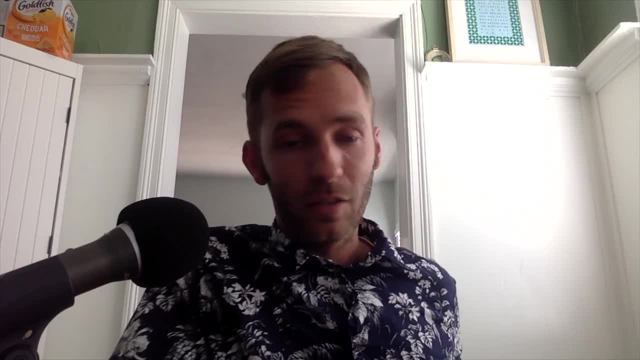 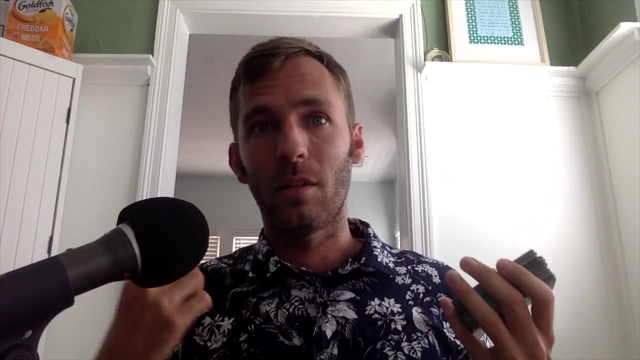 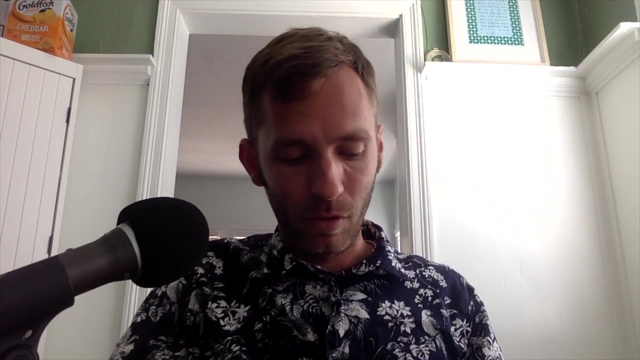 game is pretty simple and it didn't need more than that. so yeah, that's just how it works. I have another video about how to play this game, if you're interested in triumvirate, and I'll link that up here and in the description below. and but yeah, let me walk you through how the game crafters. 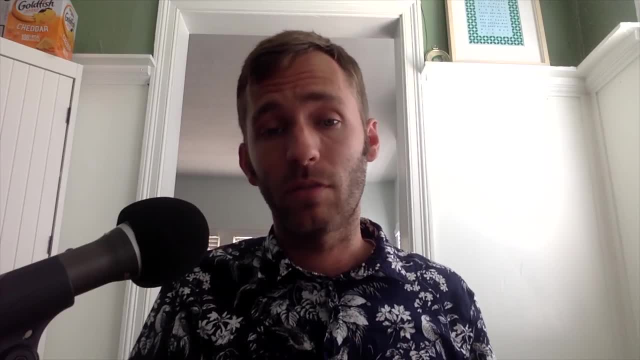 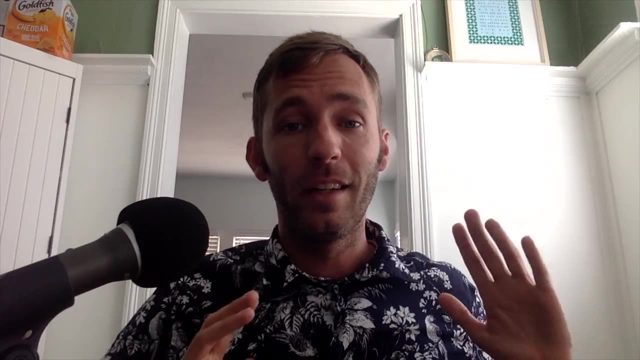 site works. it's really pretty straightforward and very user-friendly, so I'm really grateful to the people at the game crafter for creating this business. it was such a great idea. they started this. I kind of wish I had done it, but they are great to work with. 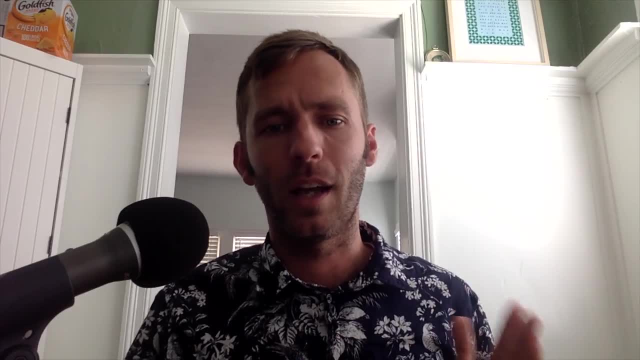 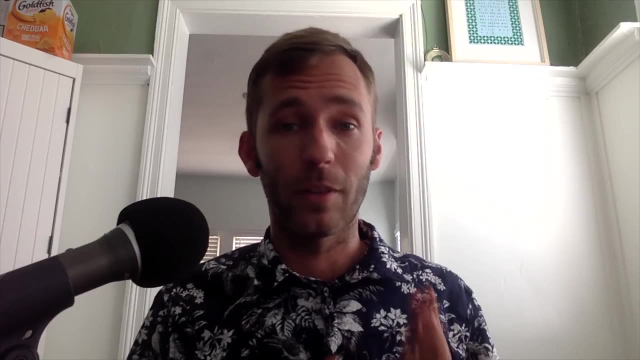 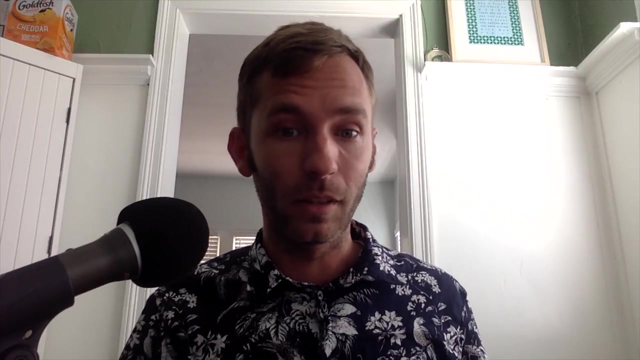 you, sometimes things can take a while to get here, but I don't. I'm not a really good judge of that, because I ordered my proof of my first card game right when we were going into the coronavirus pandemic in March 2020 or so, so that they had to shut down their thing. just you know. legally, 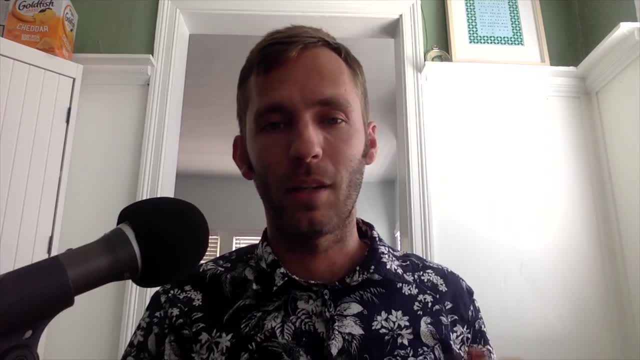 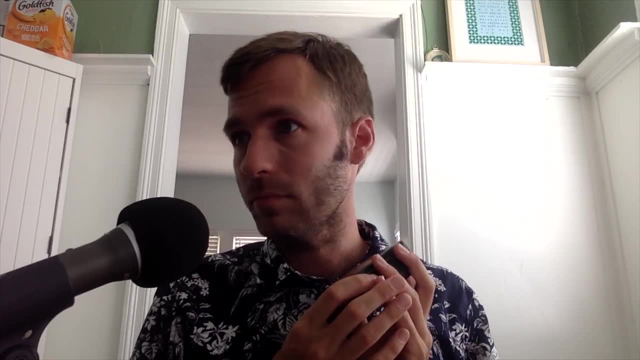 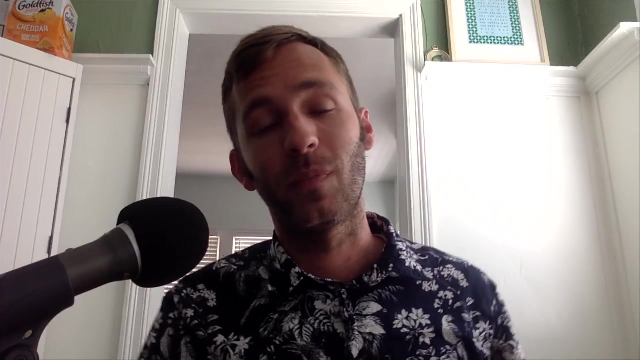 and they finally reopened and I was able to get my card game and they got it to me really fast. it was perfect. that comes actually in like a plastic, shrink-wrapped, you know wrapping, which is so helpful to keep it from getting damaged, and then that's in like a box. so, yeah, really great. 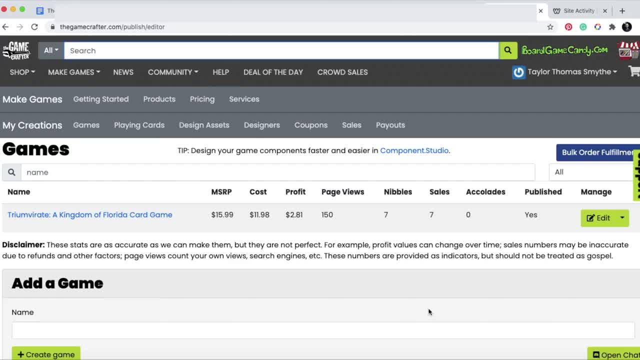 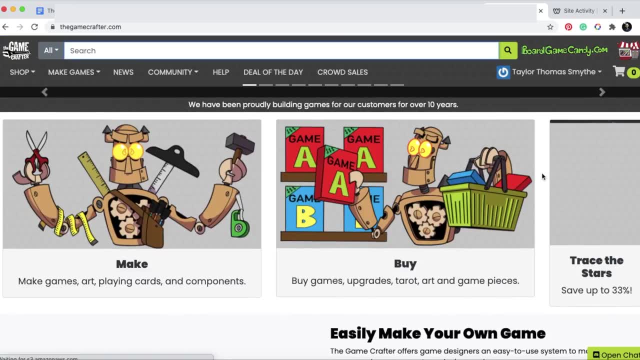 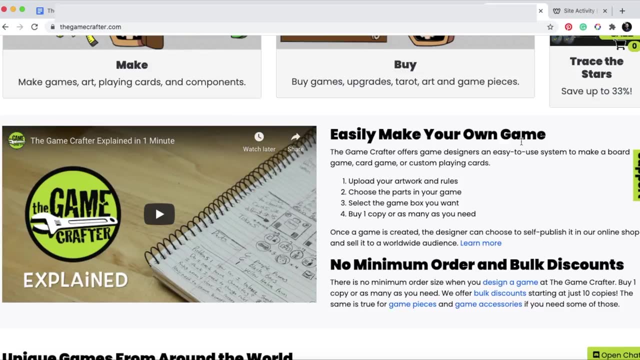 quality stuff. let me show you how it works. all right, so this is the game crafter website. this is kind of where you'll end up on the game crafter website when you first get here. like I said, they have tons of- just you know- easy, step-by-step instructions of how things work. you can also 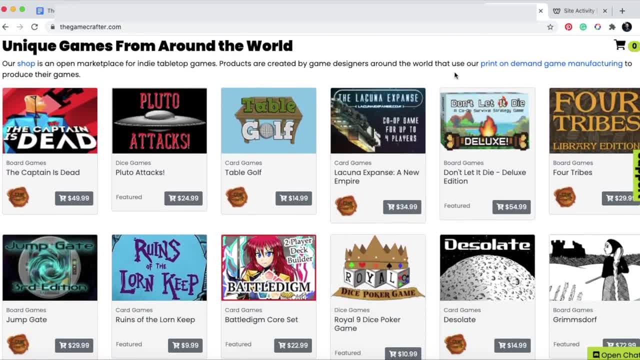 find tons of other games people have created. so if you're interested in that, you can check out the game crafter website and you can also find all the other games people have created you. what I didn't mention earlier is you can actually just you can- sell your games here and people can buy. 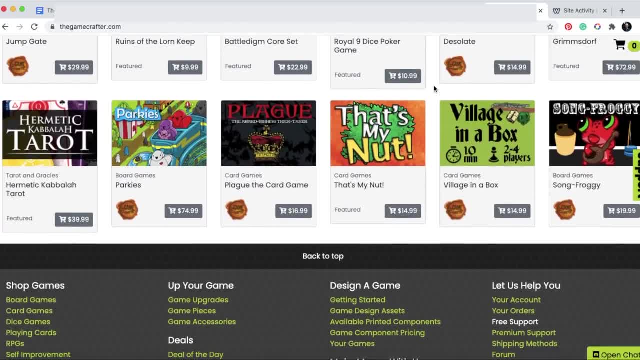 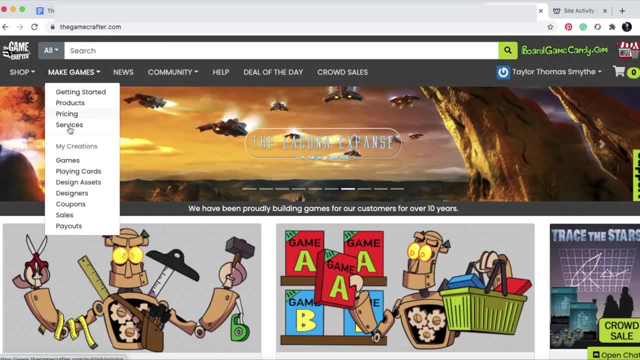 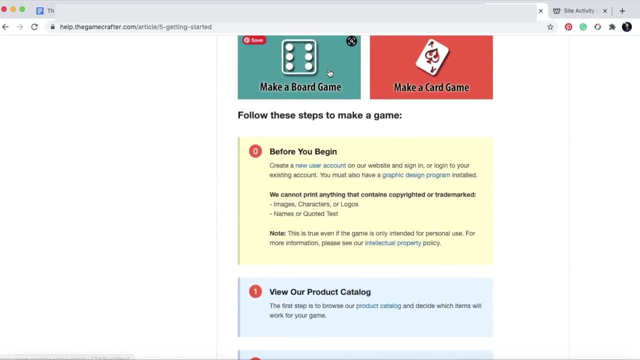 them and you can get royalties from that, which is awesome. so you can see the shop here to see all different kind of games. you can also make games. getting started is probably the place I would start. it just tells you what they do in a minute. tells you you can make a board game or a. 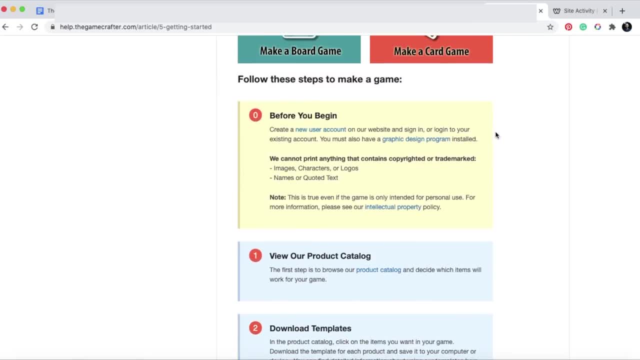 card game. you have to create an account first of all. you have to create an account first of all, so make sure you have done that. you'll import, or import input, some of your financial information if you're playing to sell these games. you also need your own sort of graphic design software. 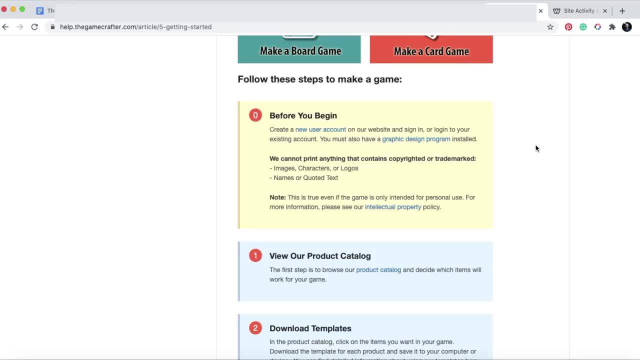 that's what they say here- to create the things that go on your cards. this is assuming that you kind of have everything. they'll give you the specs, they'll tell you how big everything needs to be- the file size, the file format, the coloring, that sort of thing. but you will create that yourself and then 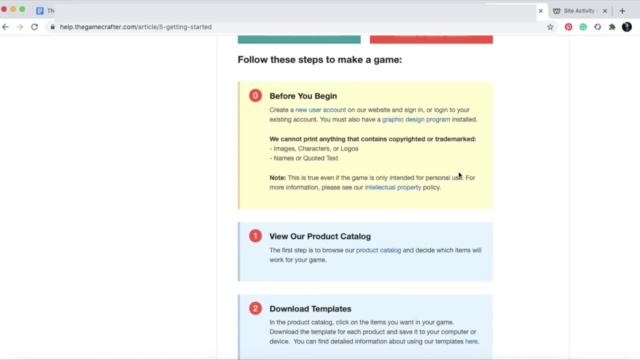 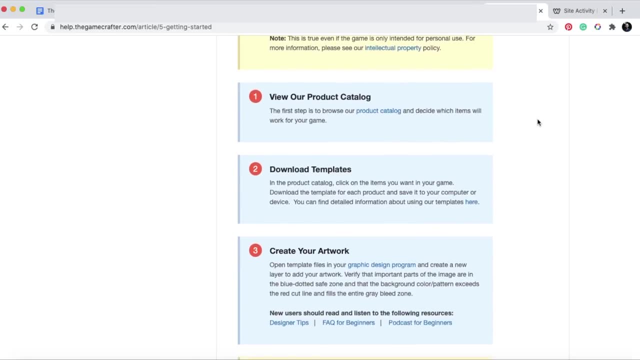 they will print it whenever someone orders it, so you can't use copyrighted things. so make sure you're not playing to do like some sort of fan game that's copyrighted for, like a you know another book series or movie series or something like that. they've got templates for everything which. 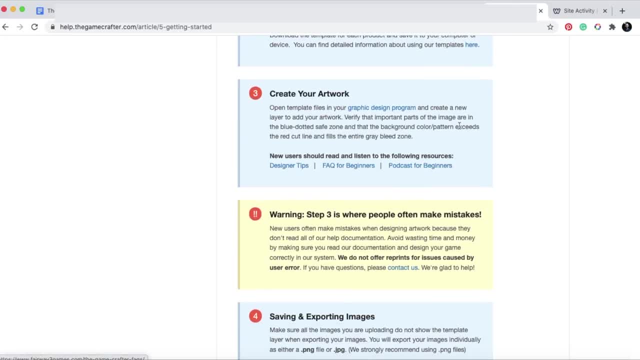 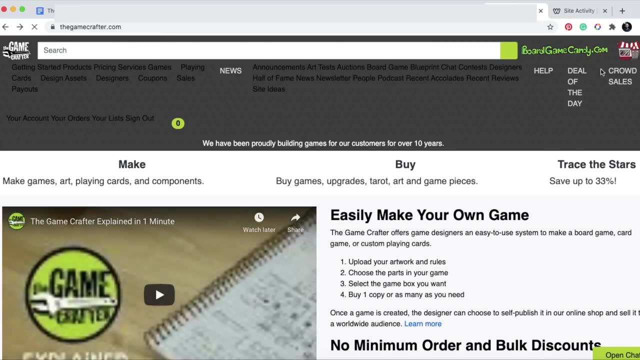 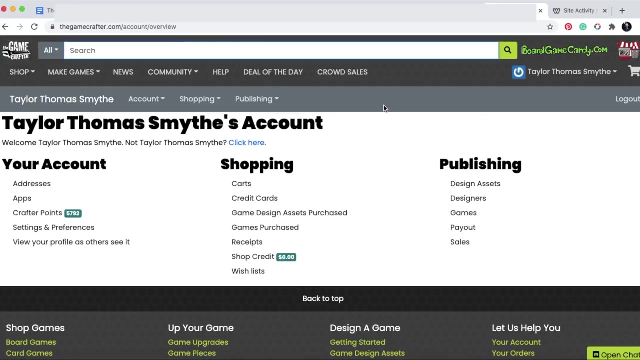 is so helpful. highly recommend using that. create your artwork, blah, blah, blah. all the stuff make a game step by step, very helpful. so let me show you what it looks like when we see a game that i've created. so we're gonna go to my account- hopefully there's nothing too personal in here- and we're gonna go to under publishing games. 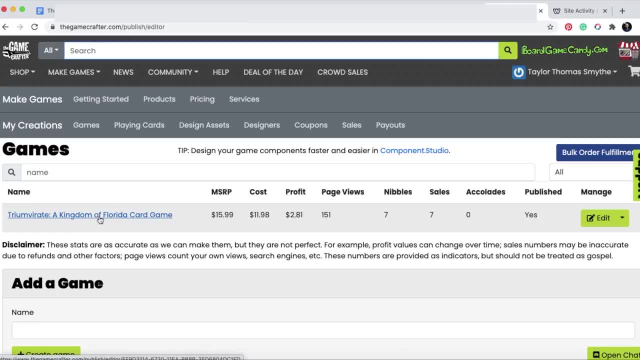 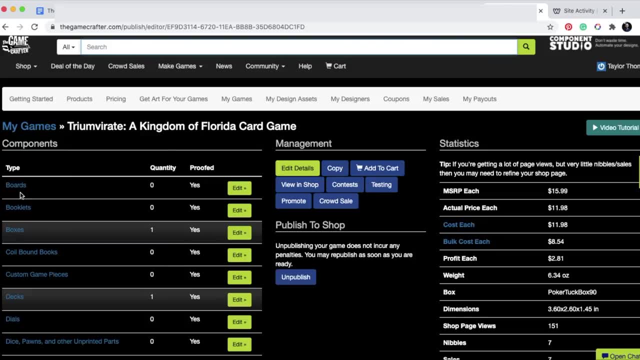 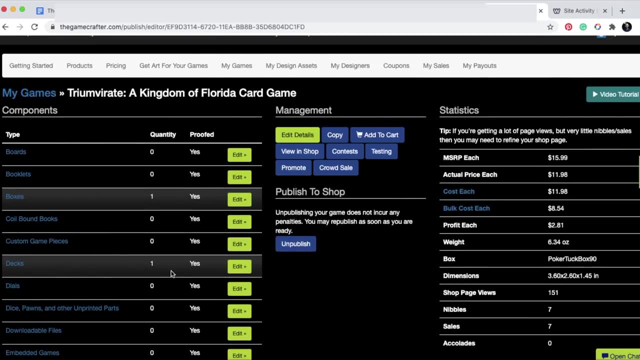 so right now i've only created this one game which i just released this week. it's called triumvirate kingdom of florida card game. in the editing section you will see what is included in this game. the only things with one quantity on it are the box. 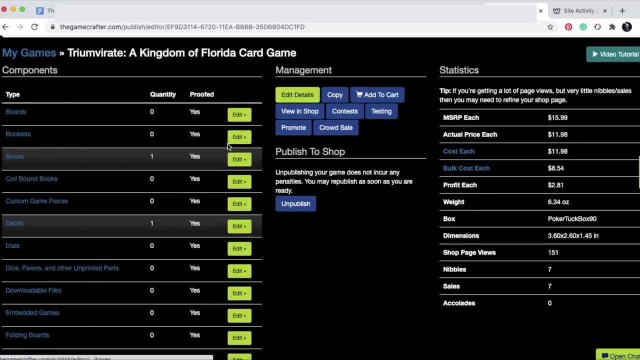 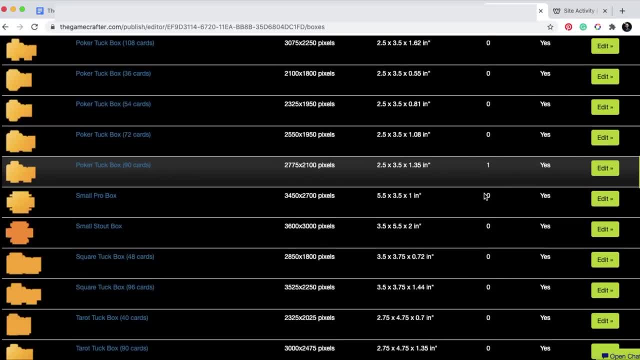 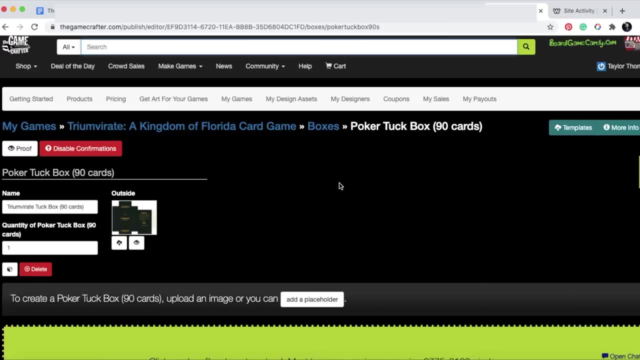 and the deck, because that's all that i'm including here. what's great is you can go click edit to see what that looks like and then scroll down to see quantity one poker tuck box. um, if i click edit to take a look at that again, it's saw it. see there. it showed all the in the dimensions and everything. 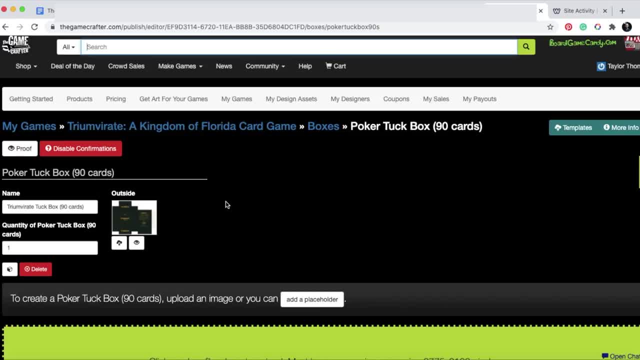 like that here. you can give it a name: um, so maybe your game has multiple tuck boxes. you want to make sure it says the right thing here, so that's all that's going to happen. so i'm going to go ahead and paste in the bottom right corner and i'm going to go ahead and pick this up and i'm going to go ahead. 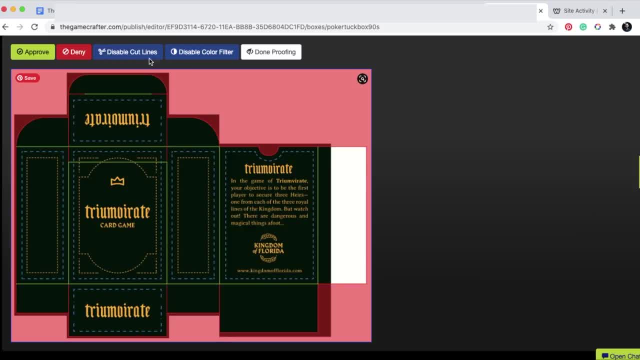 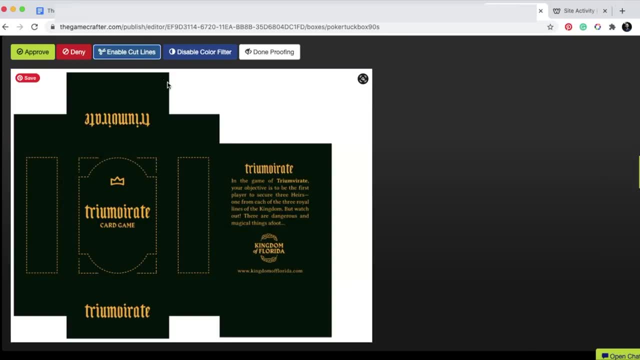 and paste it in the bottom left corner and i'm going to go ahead and paste it right here so that that's more for you to keep track of. i can take a look at what it looks like. this is great. you can see it with the cut lines or you can disable the cut lines. so the file it uploaded, you know. 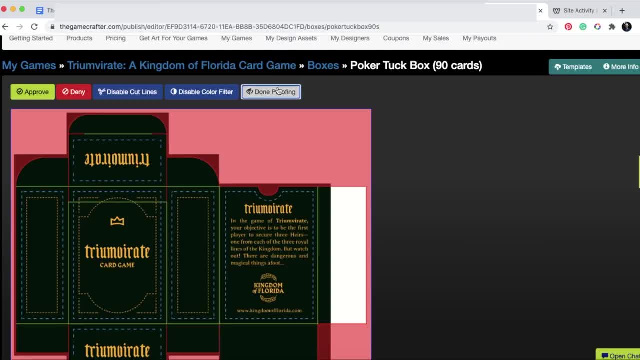 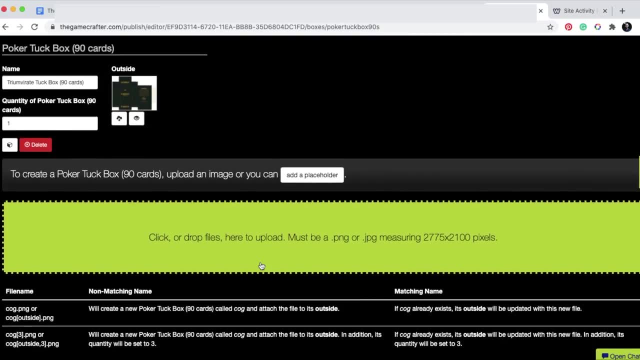 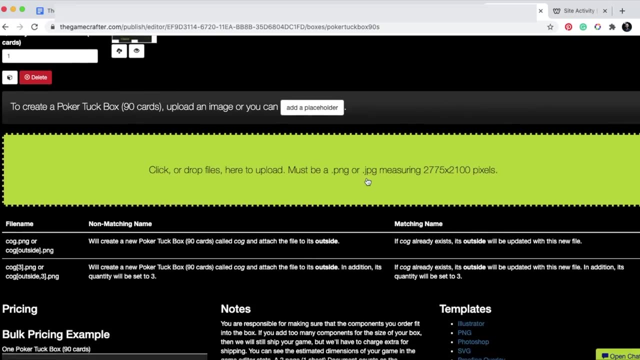 it just looked like this, but you can enable or disable and you know, click, approve or deny. it's super easy. you can download that image that you already had there. um, if you need to upload a, click here. it's super easy and it can be a png or a jpeg. i'm gonna wait for this. 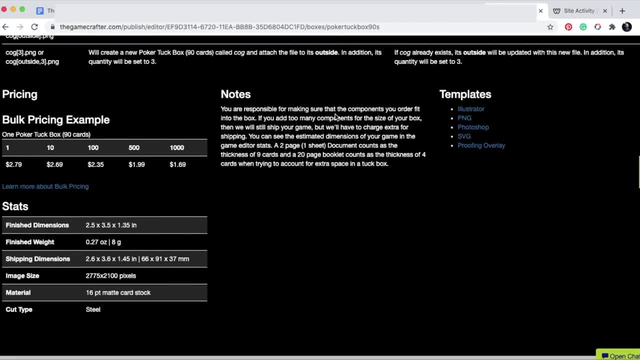 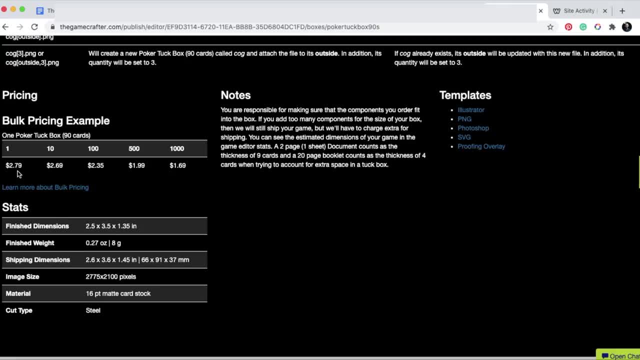 helicopter to pass over very loud. what's really helpful about the game crafter is it tells you pricing, so bulk pricing. if you bought one of these games, this tuck box itself costs two dollars and 79 cents. if you buy 10 of these, those only cost 269 a piece, and so on and so forth. if you're. 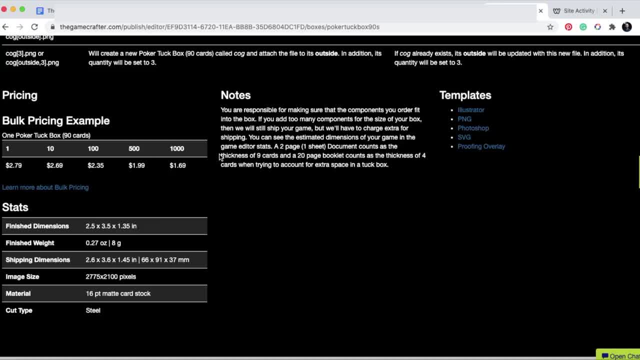 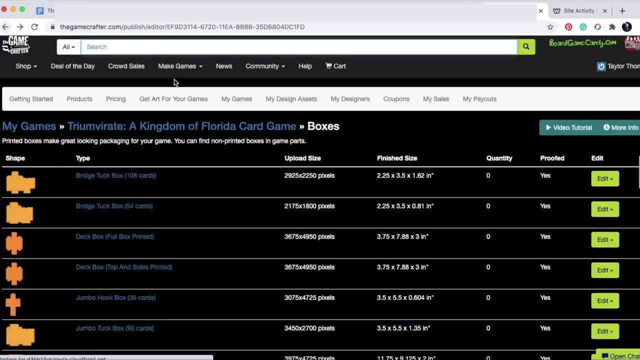 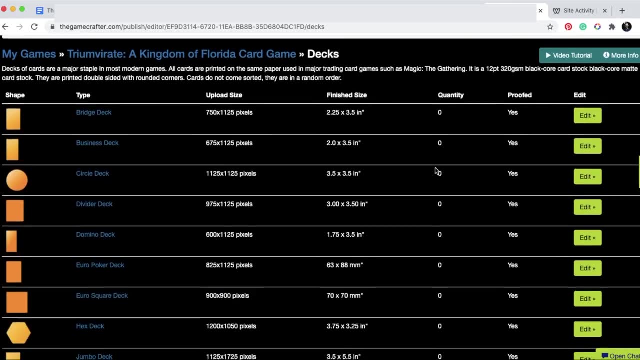 ordering a thousand. that drastically cuts it. see, it's more than a dollar a piece. that's almost, like you know, a third off the price there. um, so let's just go back um to the cards, the deck, because this is the most helpful thing to see. so i'm using a poker deck. 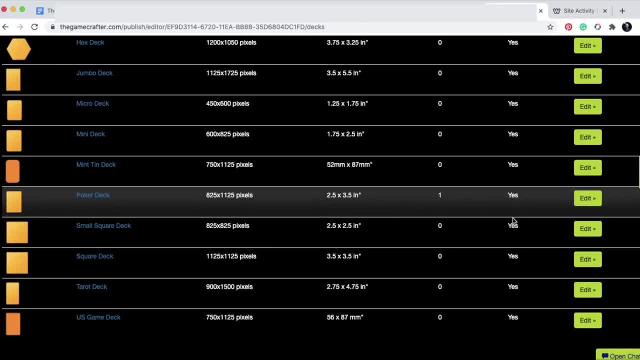 you can do different sizes of decks. you can do a hex shape deck. that's what i love about this. there's so many options. squares tells you the dimensions of that card. this is a standard size, so i want it to feel very natural in someone's hand. 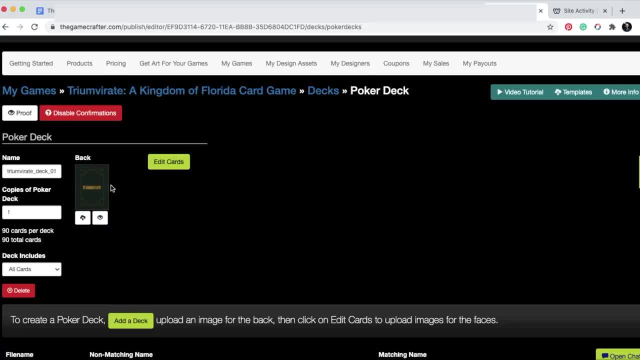 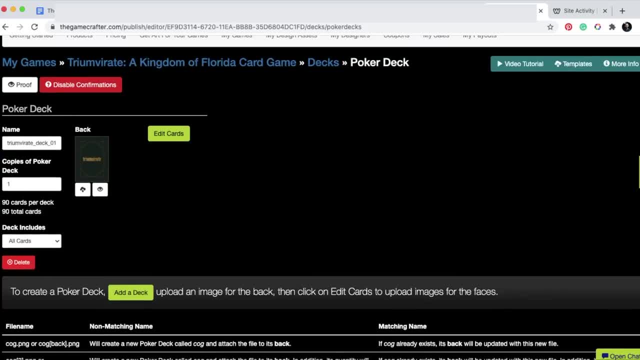 here you can click, you know, select the back of the deck. so i wanted all the backs of my cards to be the same, except for the instruction cards which i was using both sides of. but this was kind of the main thing here. i can go to edit cards. 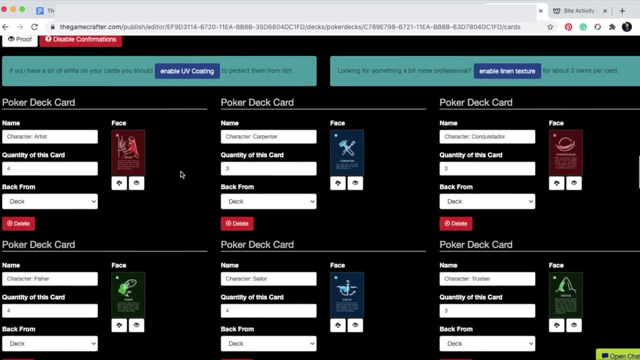 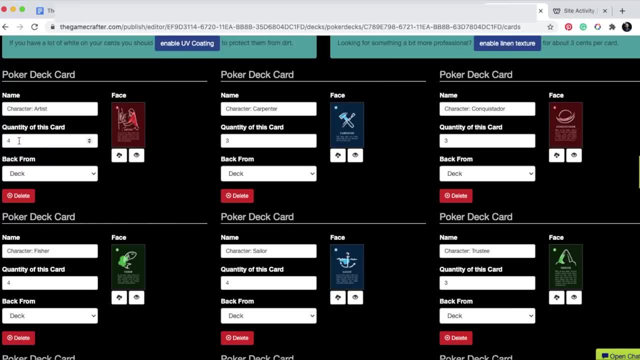 to see every single card that's in this deck and, again so easy to use. you can name the card again. this is helpful when you're kind of quickly scanning through here. quantity of this card refers to how many of the of this card there are in the deck. so there are four of this. 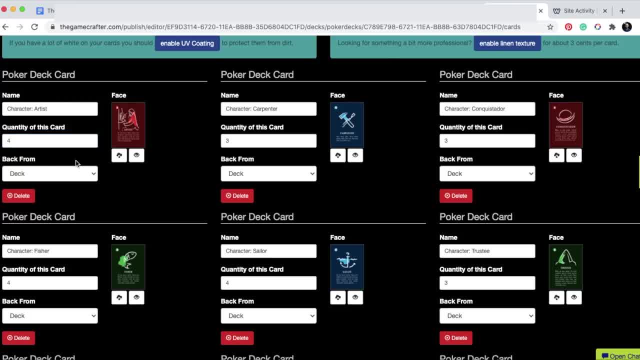 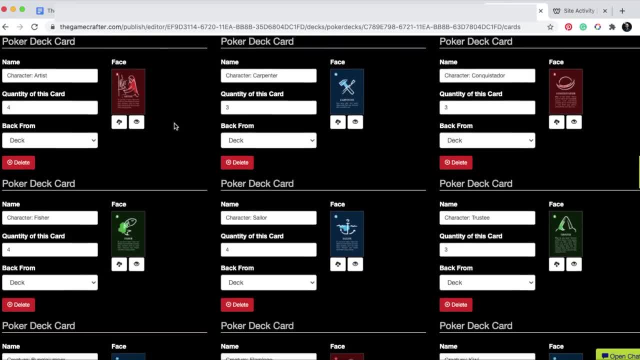 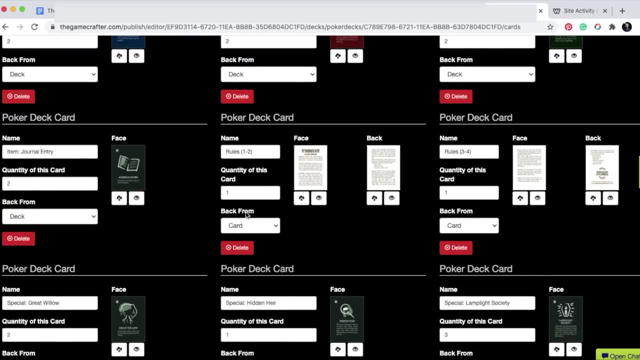 artist character card and then it says use the back from deck. so on that last page, the image that we selected for the back of the cards, that's what this one's going to draw from. that's the default. however, if i scrolled down to the rule cards, um, i'm saying use back from card, which means 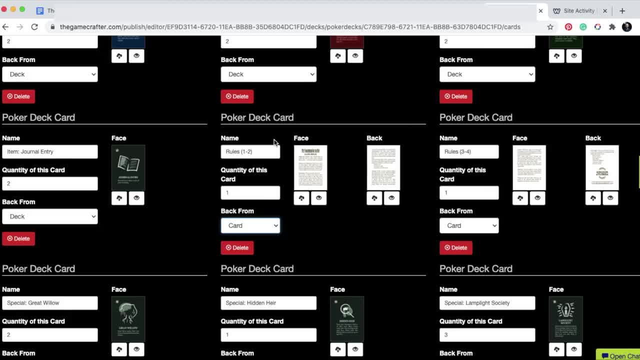 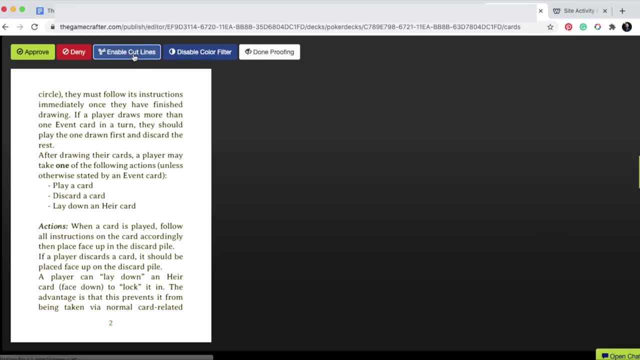 i'm going to upload my own back for this specific card, so i only did that for the rules cards here, um, and you can see what those look like again. you can see it with or without the cut lines. you upload the file with the bleed. bleed is just referring to extra part of your design. 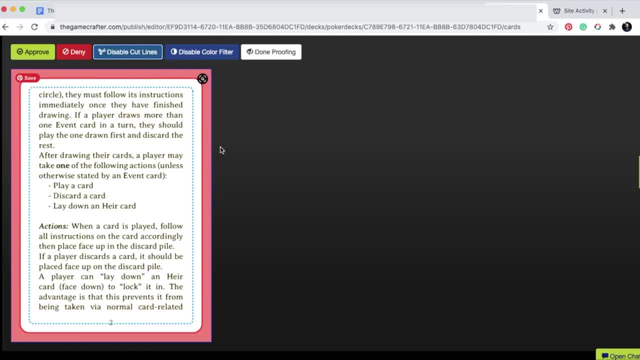 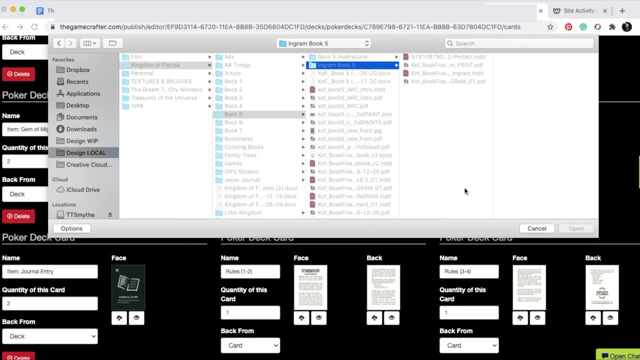 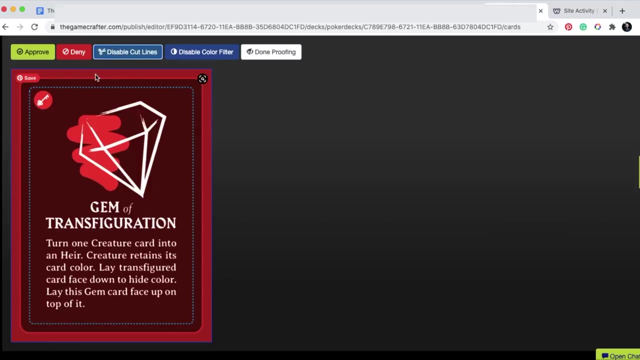 that will extend and beyond the line where they cut, just so there's not any weird extra. you know, on this card it actually is white, but if this is a colored card, you- let's look at one of these- the gem of transfiguration. oops, ah, i don't want to upload. cancel. you know, if we didn't have bleed on this? 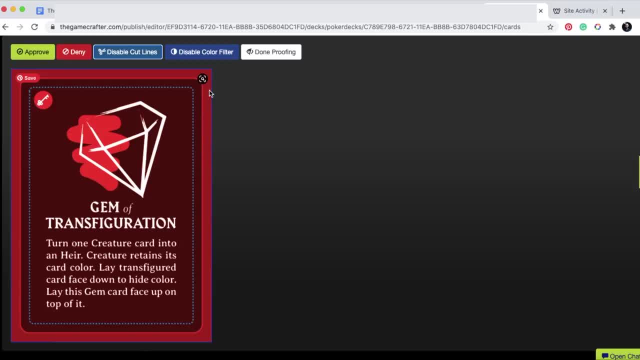 and maybe the machine didn't cut it quite exactly, because every machine that cuts the game style in this world is just kind of all white and this is just a very simple thing. but if we do cut something which is too much, you know, just like a little bit of the inside definitely. 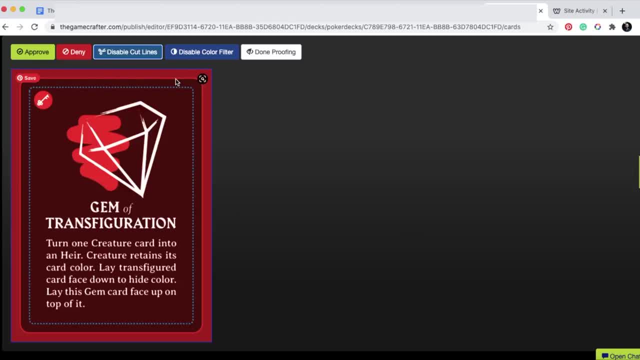 can do that. you can add another layer of layer again, but you can also add more layers if you want to. so it's not going to be perfect here and you can actually have some other things like this. like it's gonna vary, you know, by these percentages of a of an inch. um, fraction of an inch is what i'm. 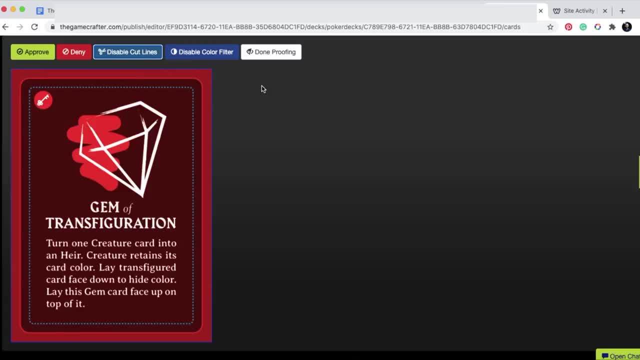 about to say so. so if that didn't have bleed in the artwork, there would be a white line around here and that would look very unprofessional. so professional stuff has bleed again. this cutline is helpful to show that you can download. this was setting my file. I set up my file to this full rectangular size of the. 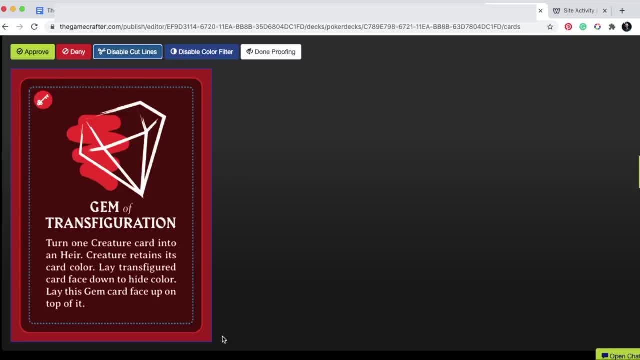 finished artwork and designed everything up to that edge. but then I use this overlay to show the red. the thick red line is where the bleed, where the card is actually cut, and then the light dashed blue line is where you want to put all of your kind of important information. you don't want any text to. 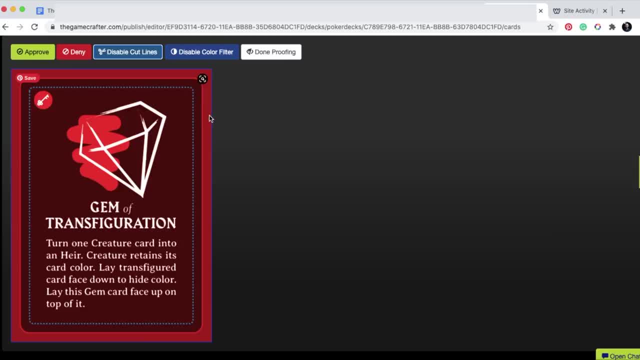 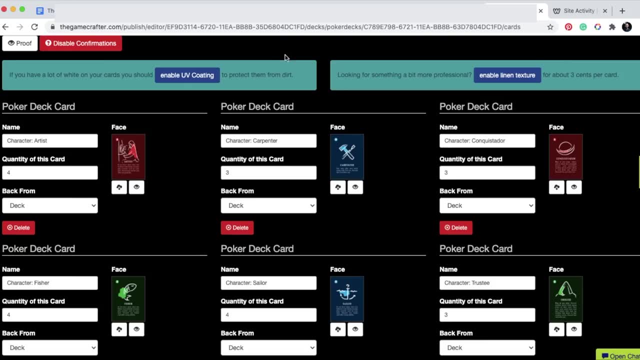 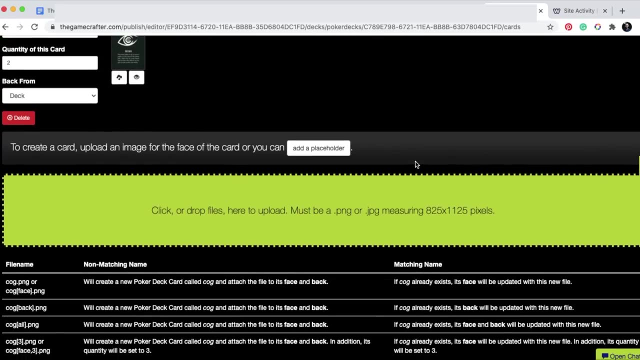 go outside of that box, otherwise that may get cut off or will look kind of weird. so that's the. they call that the trim line or something like that. sorry, someone correct me in the comments, like it's too, it's afternoon and I'm my brain is being weird right now. so yeah, you can individually upload cards. you can say: 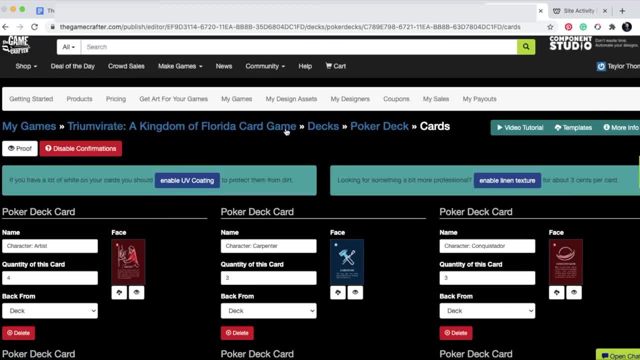 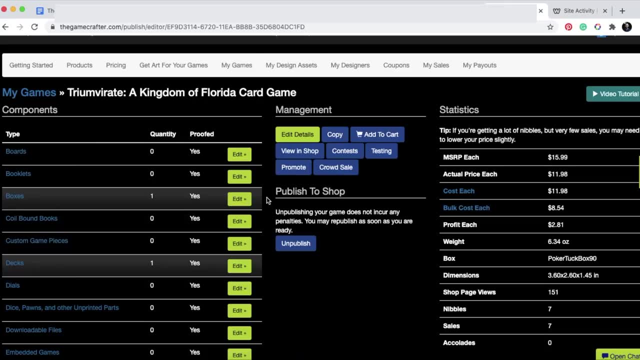 only on one of this. so very easy little. you just click on it and click, you know, whatever file you want to go there, and then it uploads it. it's very fast, it's like instant. so that's it. that's like basically how you create a card game in here. you can add other. 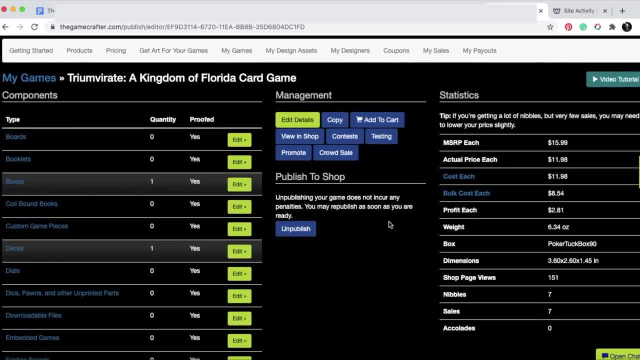 elements in here and then you can also see. you know how much are you selling it for. what's the actual price that it cost to manufacture it, what's the bolt cost? so if you ordered like ten or more of these, it would be a lot cheaper. that's a. 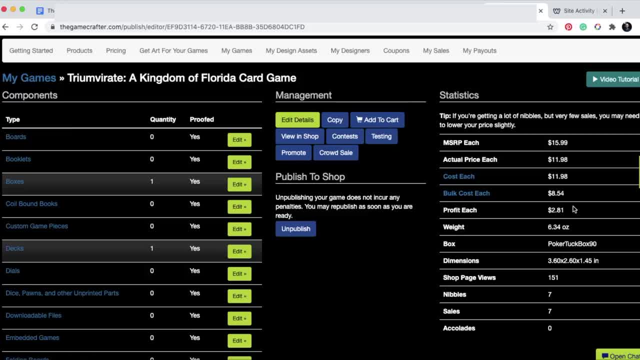 cool thing to know profit. I'm just being fully transparent here with you guys. I don't make a ton off of these games, see. I meant like make less than three dollars, but I'm okay with that because there's the cost of the materials and the cost of. 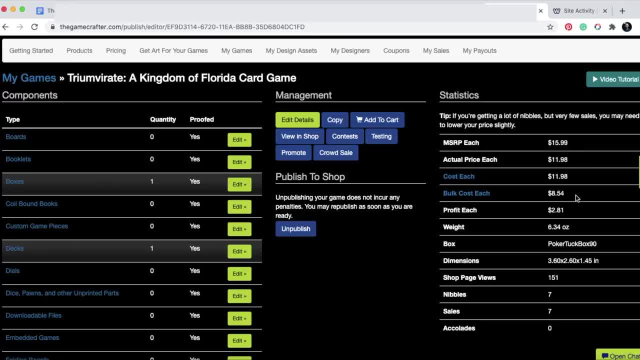 the labor to create it and ship it and the ship like all the shipping costs and stuff like that, which the game crafter handles all of that. so basically it's like they are your employees and you're paying them what for the work that they're doing and then you're getting the profit off of that without really 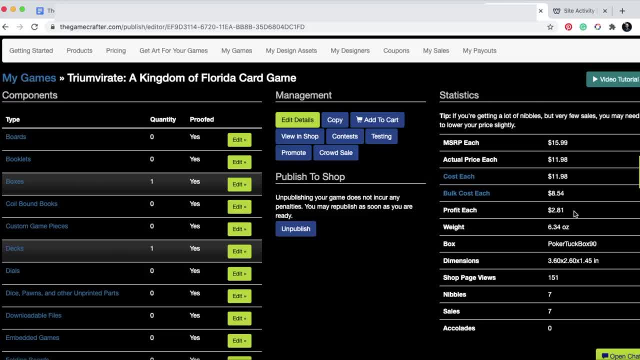 having to do any work after your game is published, except for marketing it, however you want to do so, and then you can just go ahead and just make a lot of money from it, and then you can get it back, and then you can get your money back. 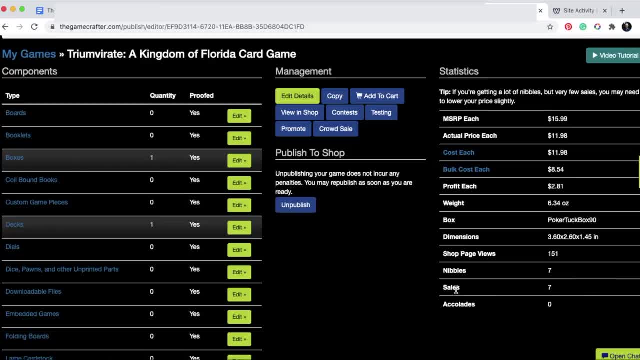 there. so that's a cool thing to know, but in my opinion that's a great thing to do quick. a few quick other things that are unique to the game crafter page views. it's not unique to them, but this shows how many people have viewed your game. 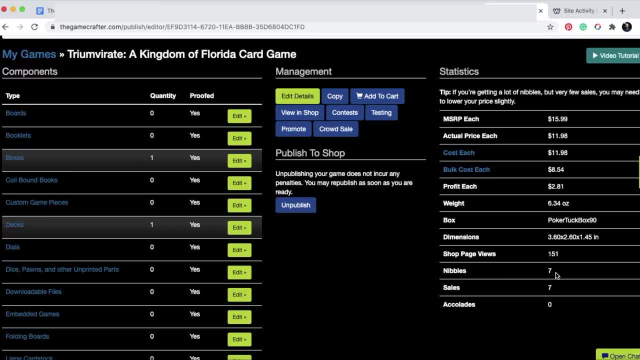 page. so there's only been up a few days. so 151 is awesome. nibbles is how many times the game has been placed in a cart. so in this case, seven copies of this game and placed in a cart, and then how many have been purchased, or seven if you. 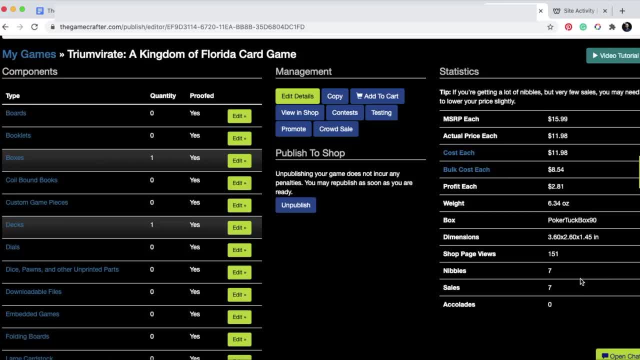 that will also show up here, so it doesn't distinguish, like, between someone else and you buying, like a your own copy of it. um, another thing to know is that you, as the publisher of the game, you will buy it and you only pay the actual price. um, since you know, if it was marked up, you would. 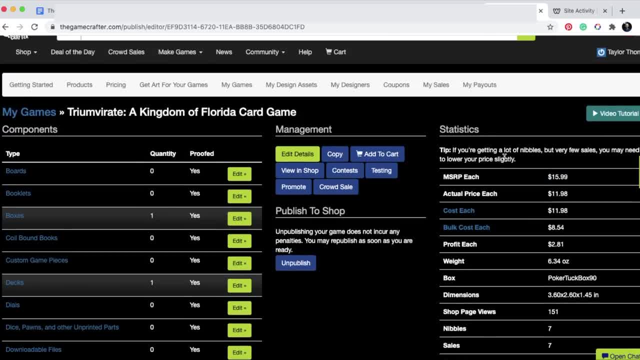 already get the profit, like the profit would be going back to you anyway. so they just charge you the like production cost, which is nice. you can view the game in the shop, um, to see you know once it's published. this would say publish instead of unpublished, there on that last page, if you. 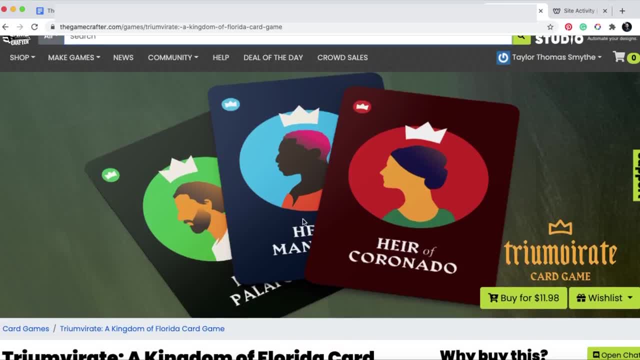 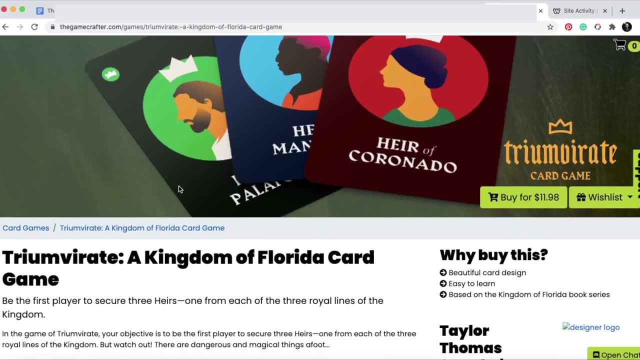 haven't published it yet and you just click publish and it'll go live, but your game page will still exist here if you- even if the game isn't live- but it'll have a little message, like mine did up until like a week ago when i made this live- had a message that said: 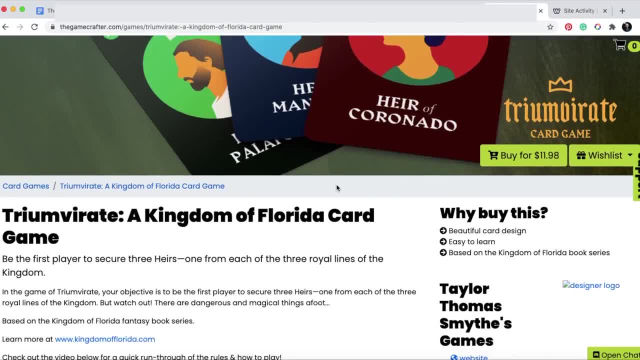 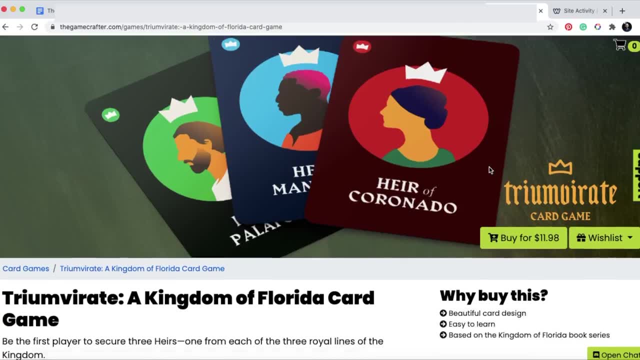 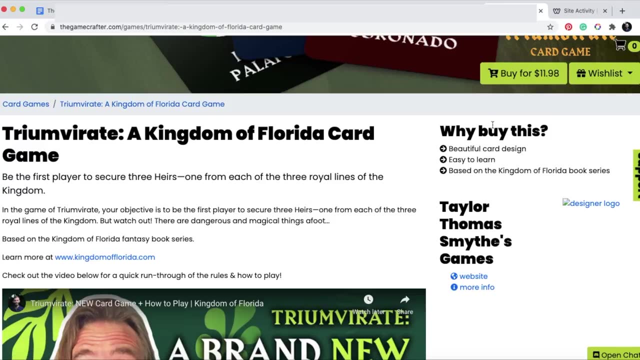 you know this game is not available for purchase right now. the the author has not made it available so you can create a header image. you can create like a game logo image that's transparent and overlays over that. your title of your game goes here. you know the category you can put in: some. 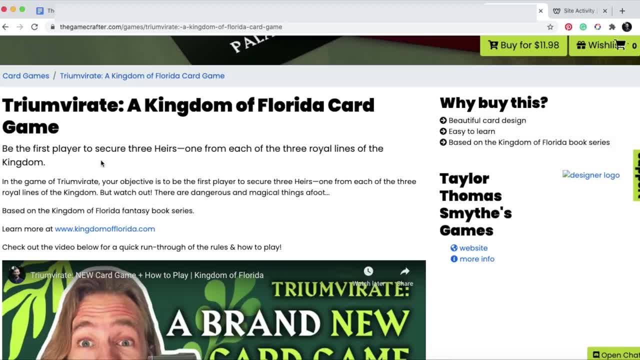 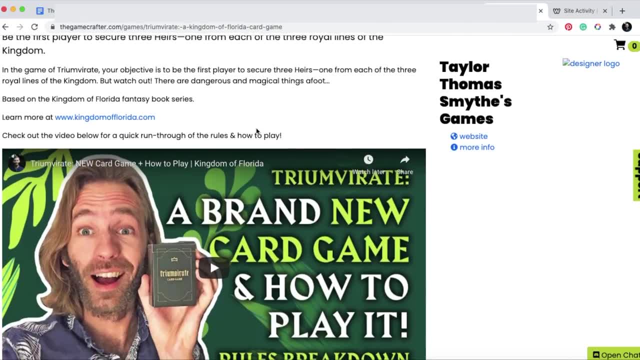 reasons why someone should buy this. a description like a one sentence description, a longer description, which you want to just tell people how to play it. um, you can put links and hyperlinks in here. i made a video of how to play my game and put in here because i thought what better way to show? 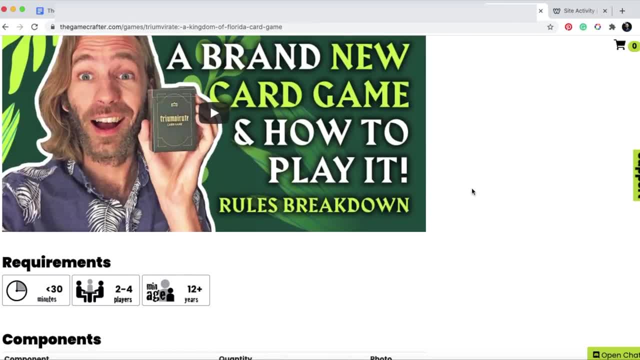 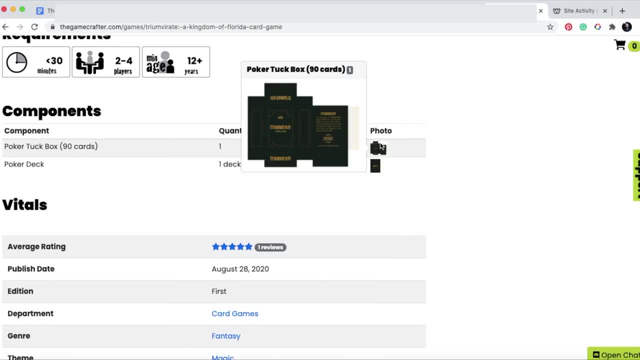 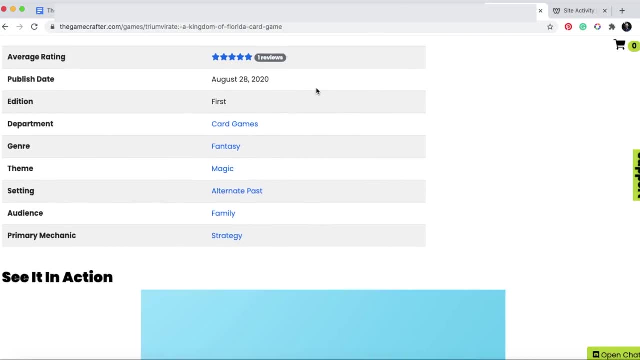 someone you know what this game is about than to actually demonstrate it. so show you what. what's included in this game: a deck of 90 cards and a inside of a tuck box actually shows the images here, which is kind of interesting but um kind of cool: the rating when it was published, genres and things you can you pick. 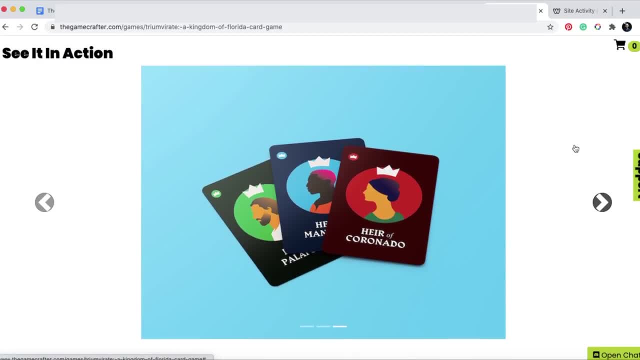 all of these things on your settings in the back. so that's great, see it in action. you can upload images. um, so this is helpful to people to see what this game looks like. um, i actually had downloaded some mock-ups that were able to be customized and include them in here. um, just so they're really. 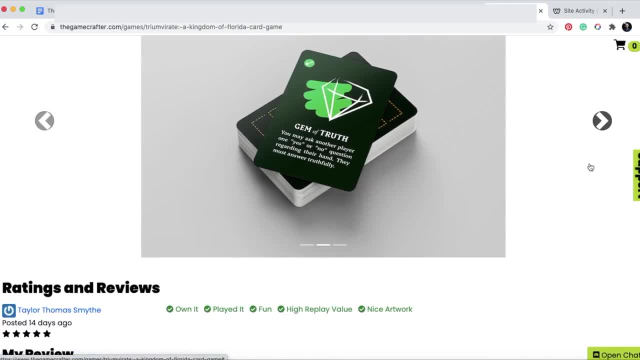 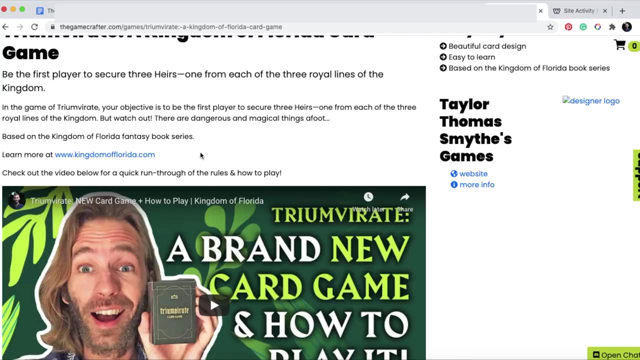 clean. you can use photos of your game or you can use photos of people playing it. um, it's a lot of great things. you- this is very like html friendly, so you can. there's a lot of code you can do like you can put probably multiple videos in here. you could put other images, other texts and links and things.